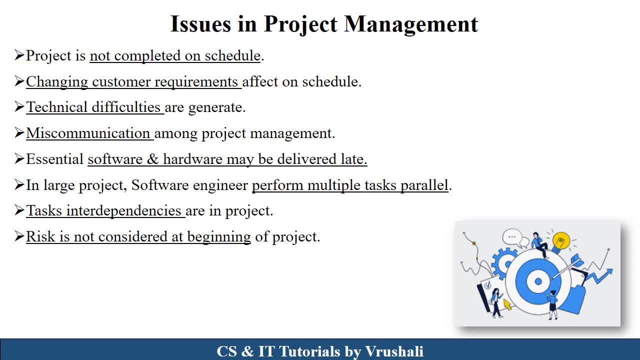 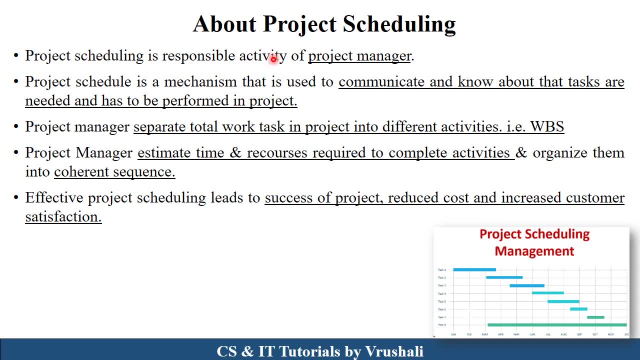 to solving all these type of issues. project scheduling is there Now let understand what is project scheduling. Basically, project scheduling this activity performed by project manager in planning phase of software development life cycle. Project manager separate your total project into different activities. Basically, they create a work breakdown structure. In previous session, 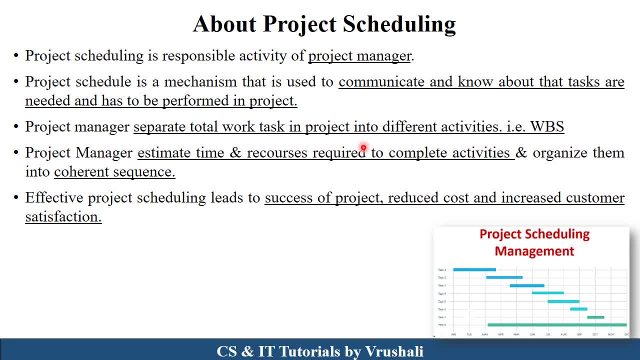 we discuss work breakdown structure in detail, For example, as a software development life cycle project manager divide your project in different activities, like requirement gathering, development testing, in this way. After that, project manager provide time and resources to each and every activity. They provide start and end date of each and every activity. So, basically, 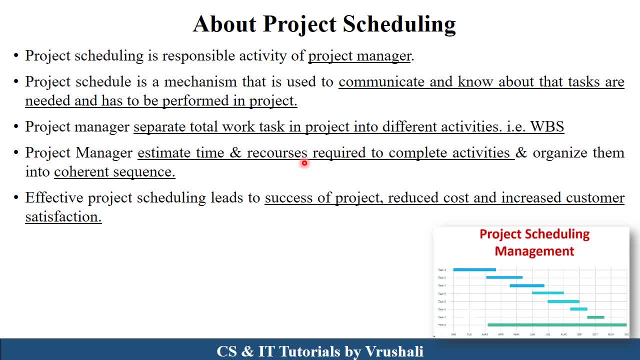 this is called as project scheduling. Project scheduling schedule your particular activity in particular time period. Effective project scheduling leads the success of project, the reduced cost and increase customer satisfaction because you deliver your project within a timeline, within a deadline. So this is called as project scheduling. 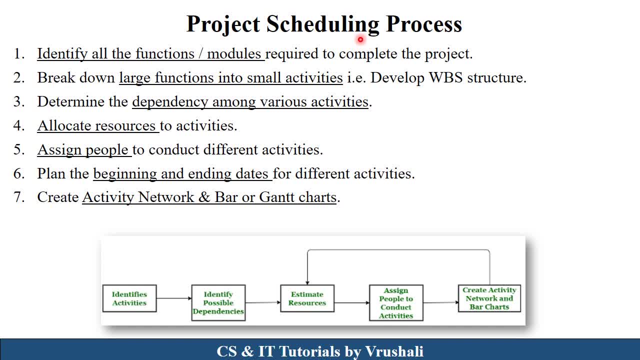 Now the next topic is project scheduling process. So firstly, project manager, identify all the modules required for completing a particular project and divide those modules into different small activities, Means as a project development life cycle. they divide a particular process in different tasks, like requirement gathering. under requirement gathering there is a sub activities like 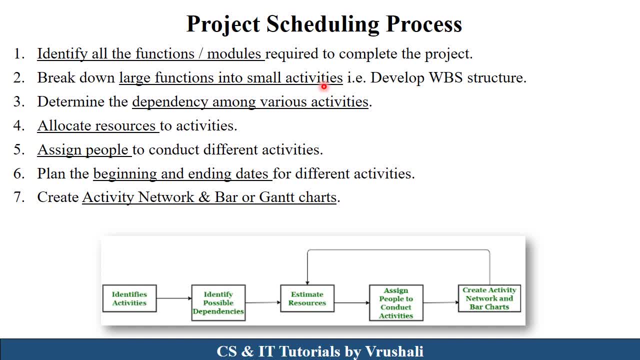 project development, project implementation, project scheduling, Then if a project manager for interview, then a survey, then a group discussion, then after that designing phase, so under design there is architectural design, structural design. after that development, then testing, different types of testing, so they divide this complete structure. after that they find out dependency. 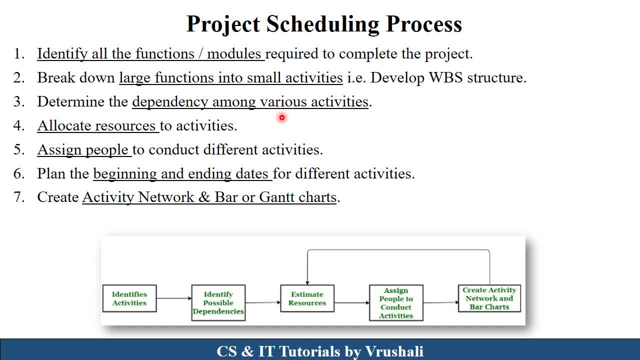 among various activities. means designer, send output to the developer team. means there is a dependency between those activities. right after that they allocated resources, like software and hardware resources, to each and every activities. then they assign people to conduct different activities. they assign particular team member for designer team, for developer team, tester team. 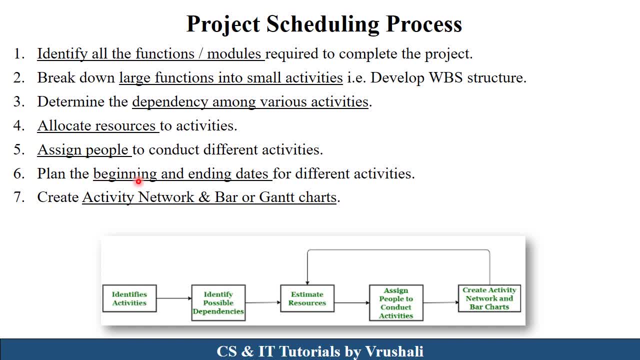 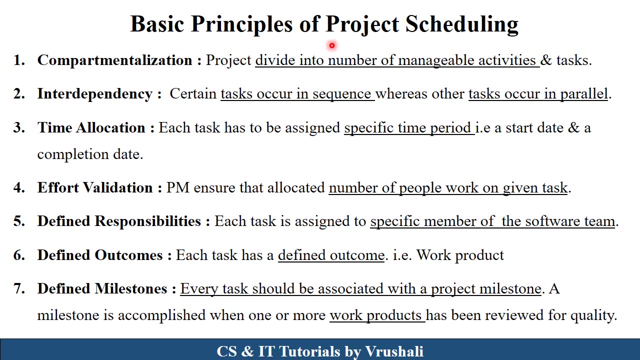 to particular project. then after that they plan beginning and ending date of different activities and after creating this all information, they mention this information in graphical format. for that purpose they use activity network or bar or gantt charts for visualization purpose. so this is a process of project scheduling. now the next topic is basic principles of project scheduling. 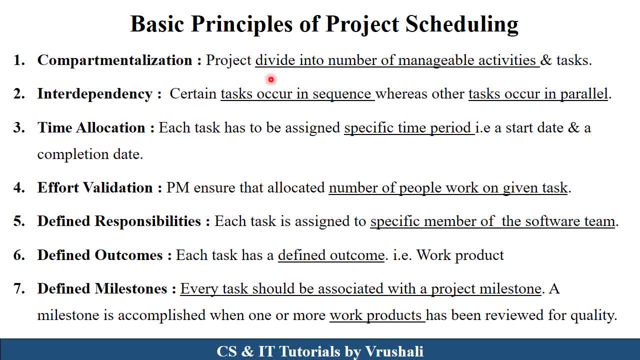 the first principle is: compartmentalization means your complete project divide into number of manageable activities. some small project required small number of activities. they require not much requirement gathering, not much designing. but when there is a large and complex project there is a detail design, detailed development is required. so according to that they divide. 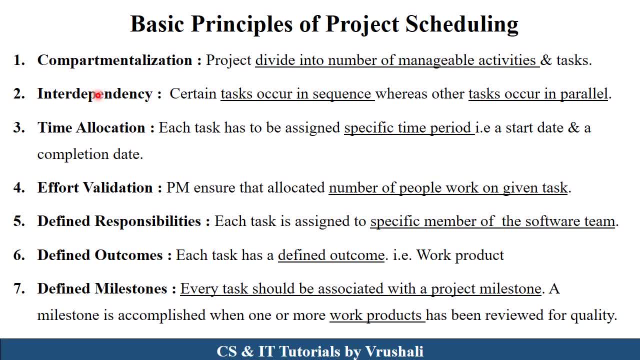 your project into managerial activities, activities and tasks. Second principle is interdependency. They find out which tasks occur in sequence or which tasks occur in parallel. Next one is a time allocation. So project manager assigns specific time period, the start date and end date of each and every. 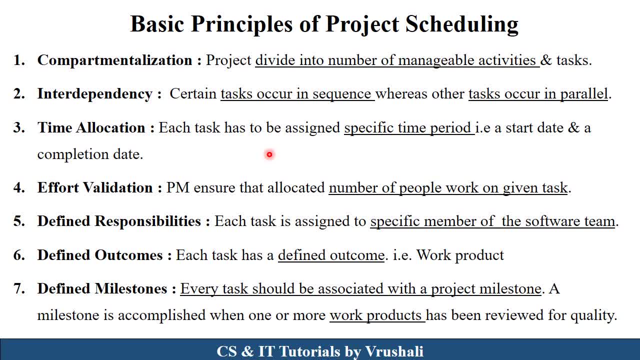 activity: When design phases start, when design phases end, after that when development phases start, and their end date. So they mention start and end date. Next one is a effort validation. So basically, project manager allocate number of people for performing a particular task in. 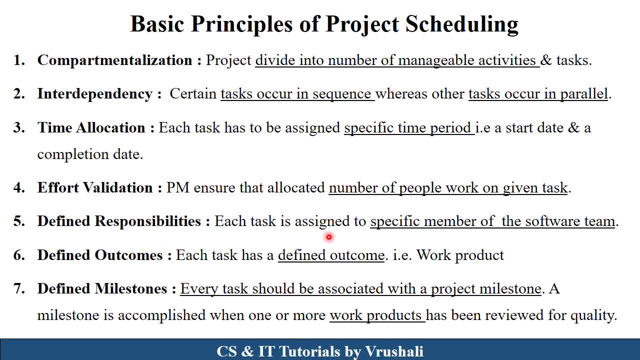 particular team. Then define responsibilities, So every software team having a particular responsibilities according to the phase of software development life cycle. Then define outcome- See every phase having a particular outcome: Requirement gathering phase having a outcome that they collect the requirement and mention in SRS document. Then designer team also. 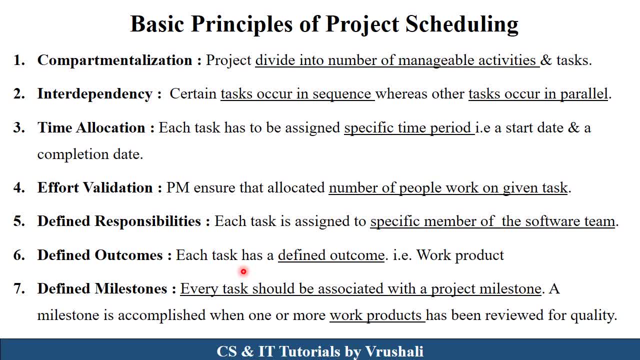 having a particular outcome. They mention overall design flow of particular project in this way. So every outcome mention in particular phases and send forward to the next phase, Then define milestone. So basically every task should be associated with project. milestone Means after completing every phase, they take a customer. 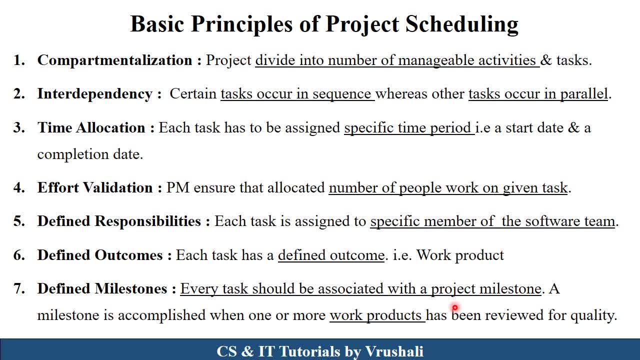 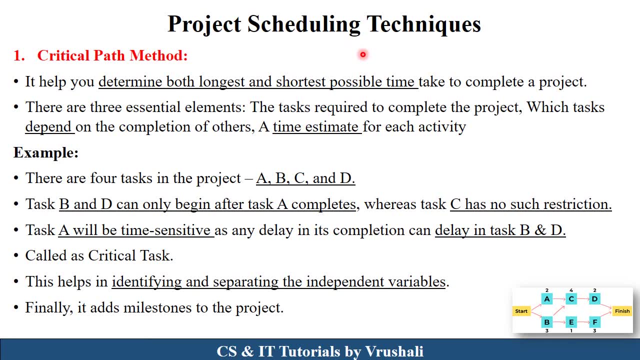 feedback from there. They check that whether it is quality or accurate output is generated or not. So after acceptance of customer, project, milestone is there. So these are the principles of project scheduling. Now the next topic is project scheduling techniques. Basically, there are total five project scheduling techniques. The first one is a critical path method. So 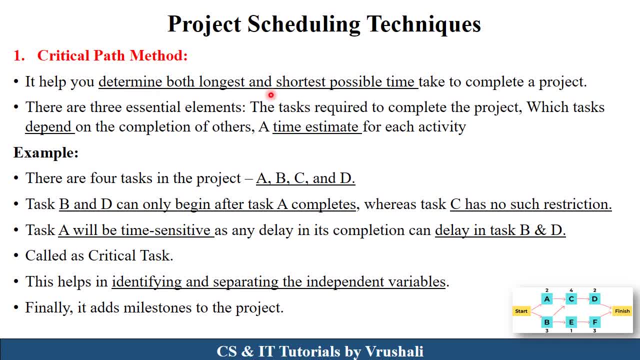 basically, this method is used to determine both longest and shortest possible time for completing a particular project. They check interdependency between the task and allocate the time according to this. Let's take the example. Suppose in particular project there are four tasks like A, B 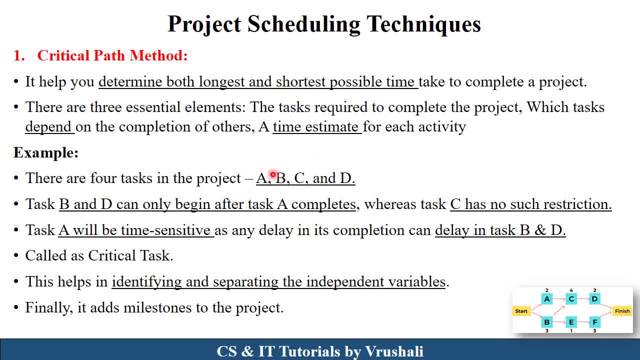 C and D. Now B and D, these two tasks have performed only after completing A task, Right. And second thing is C task have performed anytime, There is no any restrictions, Right. But suppose while performing the task the A tasks get delay due to some reason. So at the time B and D. 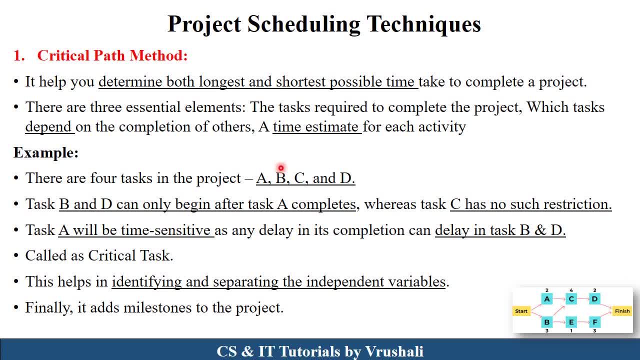 these tasks also get delay Because this B and D tasks completed only after A task, Right, So this is called as critical task. So this is a responsibility of project manager: identify and separate independent task or independent variables and assign time according to this. 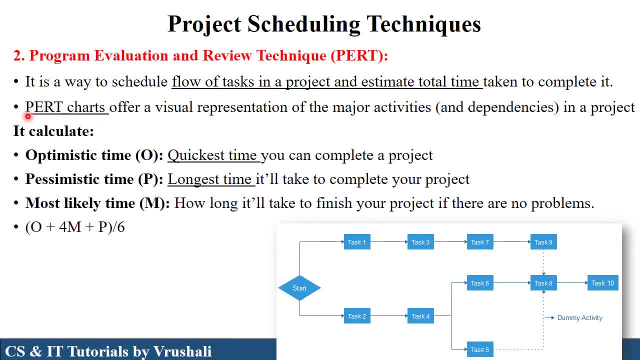 This is called as critical path method. The second method is program evaluation and review technique. Basically, project manager schedule complete flow of task in particular project and estimate total time required for particular project. For that purpose, PERT charts are used for visual representation purpose. 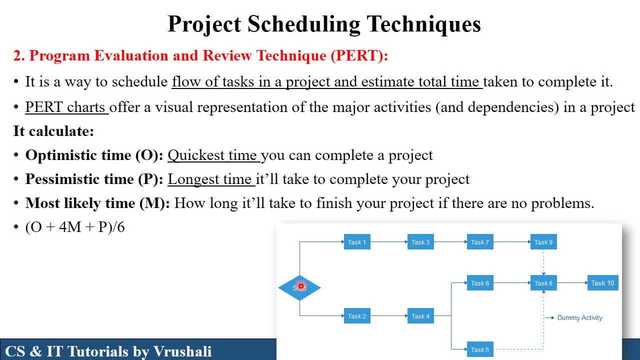 See here in this diagram. this is a PERT chart. where is a start after start. task 1, task 3, task 7 and task 9 are performed. So this is a serial transaction or sequential. this task are performed. These tasks are depend on with each other right. 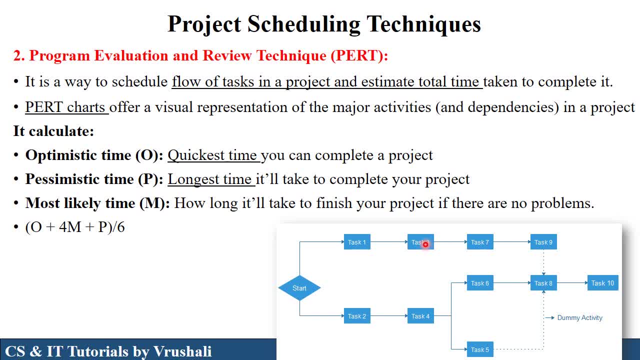 This arrow shows the how many tasks are performed and after completing which task. which task have performed? Then next one is a task 2, task 4, task, So task 6 and task 5. they are not dependent on with each other, right? So basically they identify dependencies between different activities and PERT method calculate. 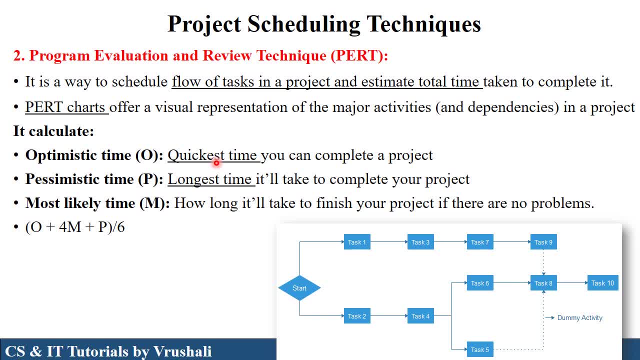 optimistic time like quickest time for completing a particular project. pessimistic time means longest time required for completing a particular project, and most likely time means how long it will take to finish your project. So, after calculating this value, this value put up in this equation- 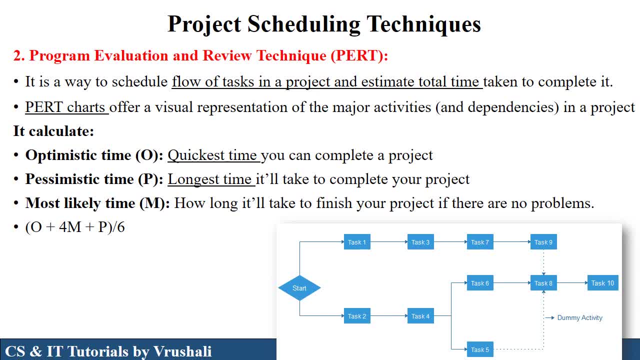 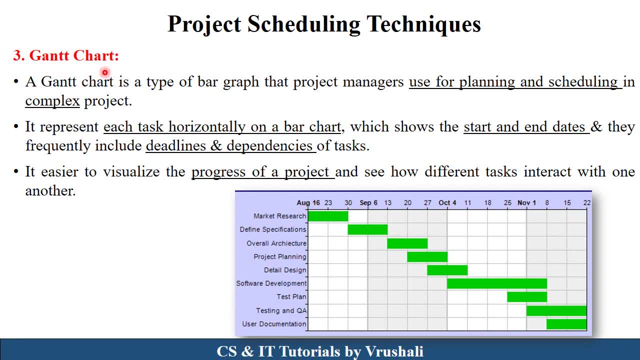 So they calculate a overall time required for completing a particular project. Now the second and most popular technique is Gantt chart. Basically, project manager use Gantt chart method for planning and scheduling a complex project purpose. See here in this diagram. here there is a market research. this is a first activity. 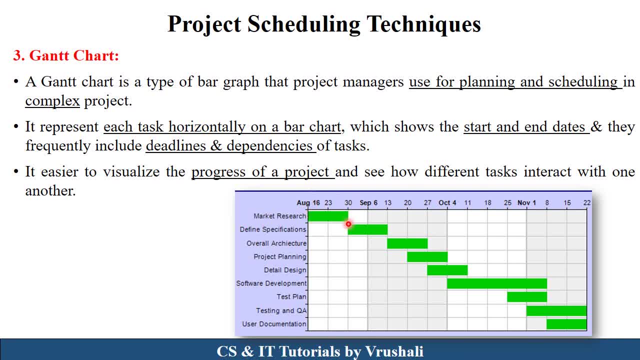 This activity start at 16 August and end at 30 August. So they show by using horizontal bar chart. is there? They mention start and end date of particular activity. Second activity specification: So this activity start at 30 August and end at 13 September. in this way, 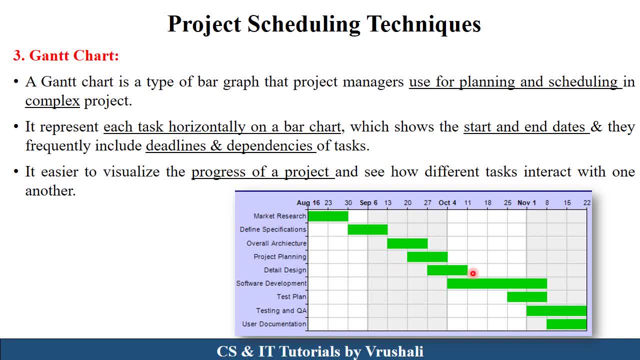 So similarly all these activities have performed and their start date and end date have mentioned. They also mention dependencies, See here, suppose design: this design phase has started 27 September, end at 11 October, But at the same time in between that development also have started, right. 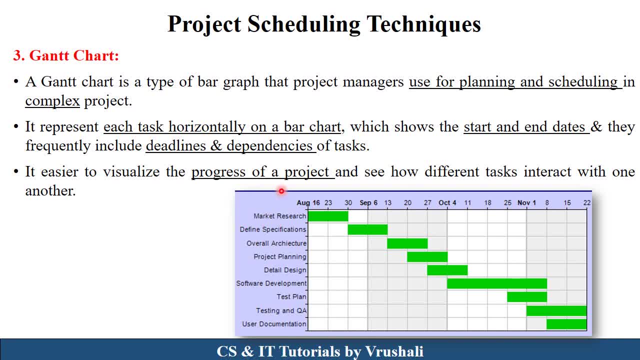 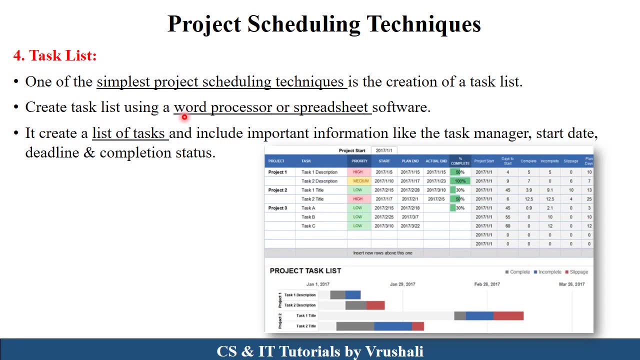 So this is a dependency. So basically is visualize the progress of project, their start and end date and complete deadline of particular project. means project have started at 16 August and end at 22 November, right? So this is called as Gantt chart. The next technique is the task list. 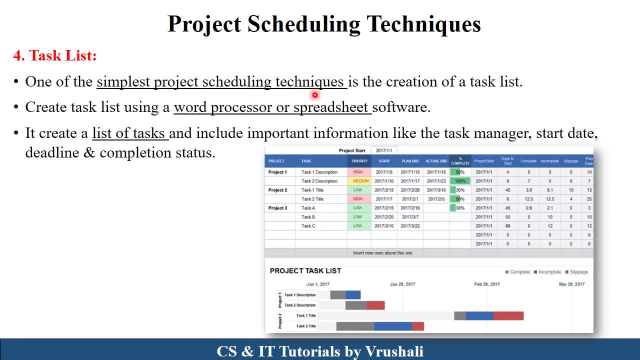 So task list is a very simplest project scheduling technique They created by using word processor and excel or spreadsheet software- See here in this diagram. So basically they create all this information In tabular format. first there is a project name, There is a task. 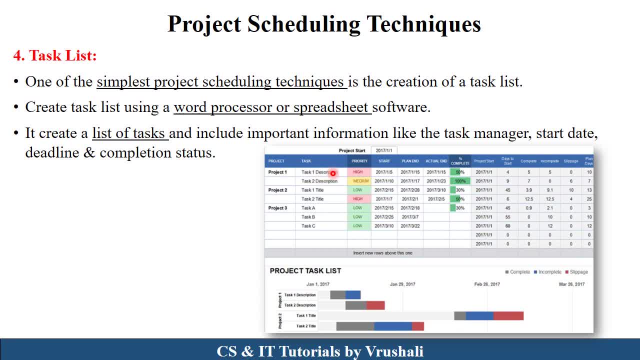 For example, this is a project one. There are two tasks like task one, task two. So task one having the highest priority for development purpose and task two having medium priority. then their start date, plan date, actual date and how many work. how many percent work have completed. like 50% task have completed. 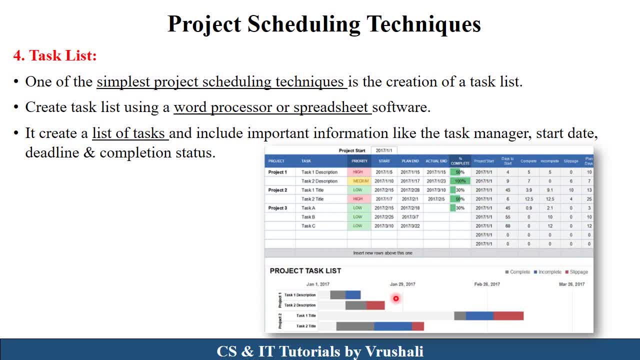 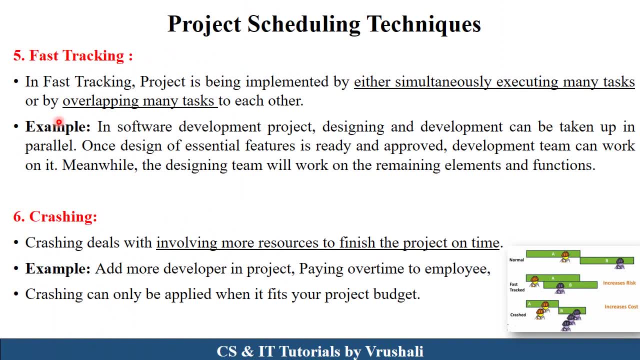 This is the 100% task is completed and this information shown in graphical format in this way. This is called as task list. Now the next technique is fast tracking and crashing. So basically, fast tracking means for completing your project within a deadline. for that purpose, 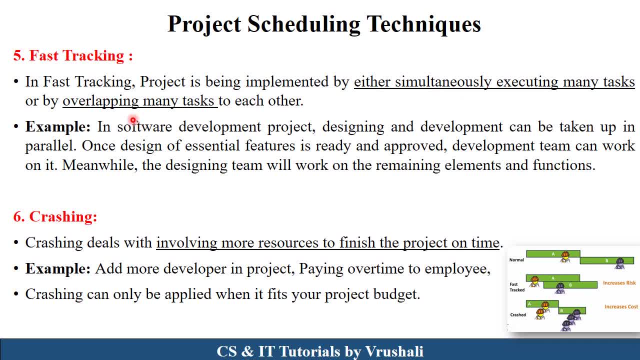 some work simultaneously have occurred, or sometimes overlapping is there. Just take example: in software development, project designing and development, These two phases occur parallelly. first designer design- a essential features which is ready. And then designer design- an essential features which is ready. And then designer design- an essential features which is ready. 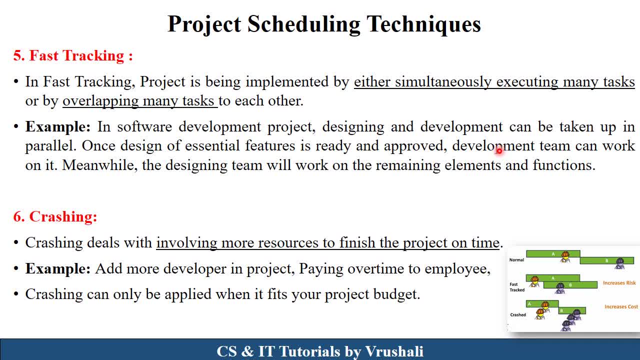 And then designer design an essential features which is ready And after that approved by the customer and sent to the development team and development team start their development work. But meanwhile designer team work on another remaining elements, See here in this diagram. So first is the a means design phase and after some designing have completed development. 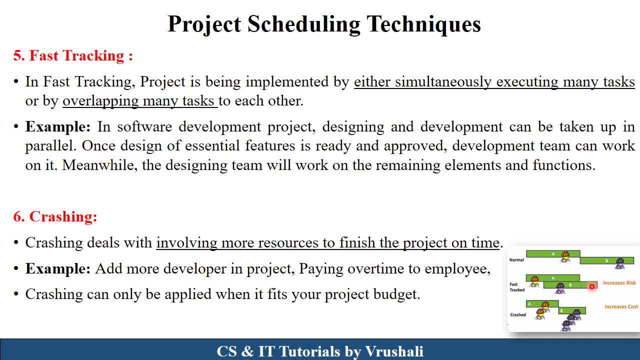 have started here. Now development have worked here, So this is called as fast tracking. parallelly, some phases have occurred. Now next one is a crashing, So crashing means More than one resources are used in particular project for completing a particular project on schedule within a deadline. 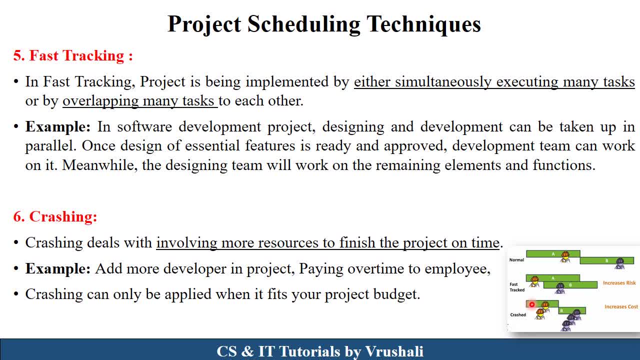 For example, see here in this diagram- This is a particular design phase and this is a development phase. So there is a more than one employee is required for completing a particular phase. So add more developer in project paying overtime to the employee. So this thing only possible when it fits your project budget. 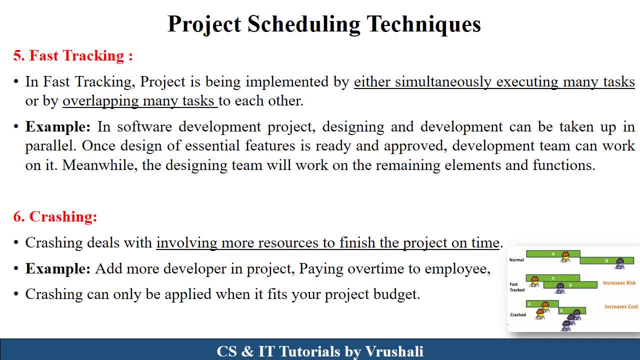 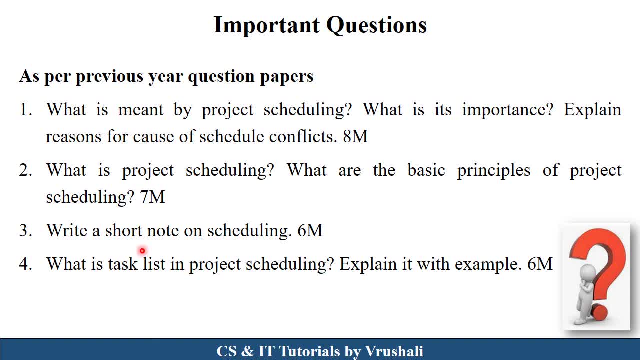 So this is called as crashing. Add more resources for completing your project within a deadline Now, as per your previous year question paper. this- all questions is important, like: what is mean by project scheduling? their importance? explain reason for cause of schedule conflicts for 8 marks. then what is project scheduling? their principles for 7 marks. short note on: 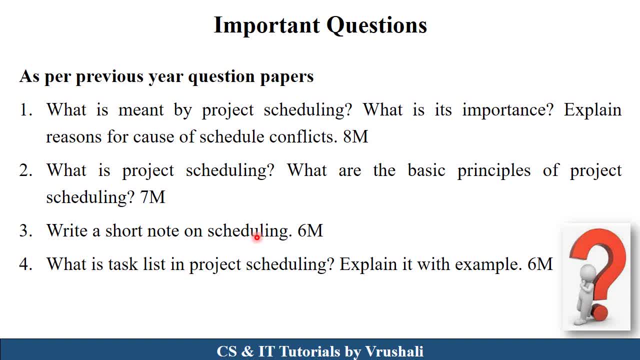 scheduling for 6 marks. here you have to mention scheduling their principles, their importance and their techniques. Then Use task list in project scheduling. explain with examples. So you have to prepare this topic completely. thank you, keep learning.